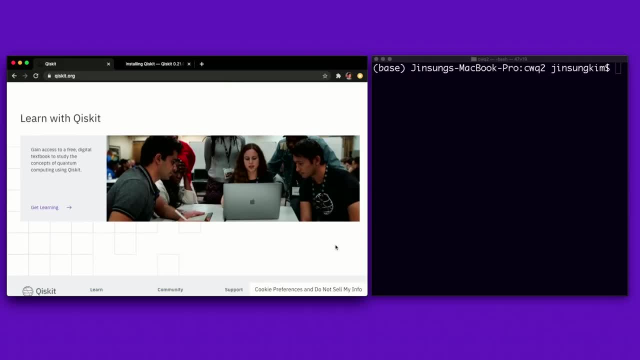 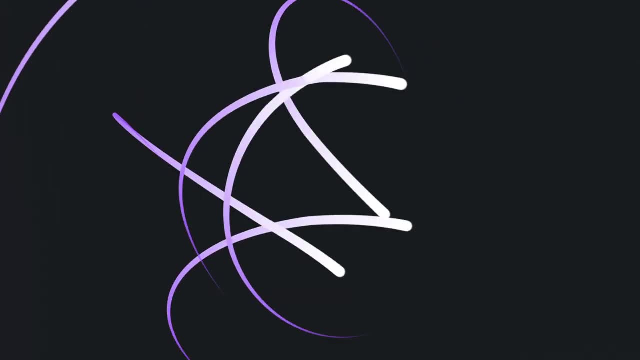 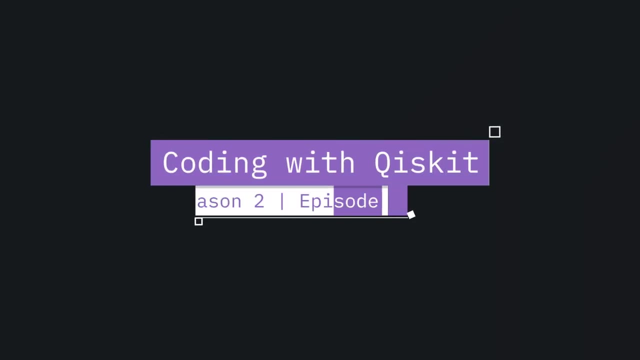 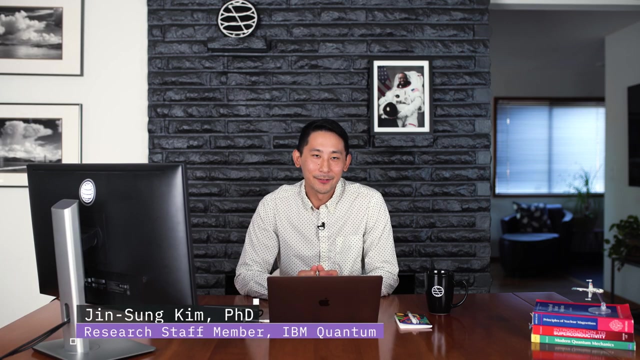 Hey, if you scroll down slightly further, there's a picture of me. Welcome back to Coding with Qiskit. I'm your host, Jin, If you're new to the series. we cover topics in quantum algorithms each week, so be sure to like and subscribe. 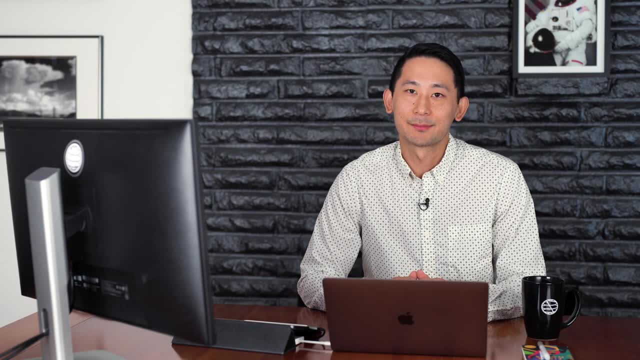 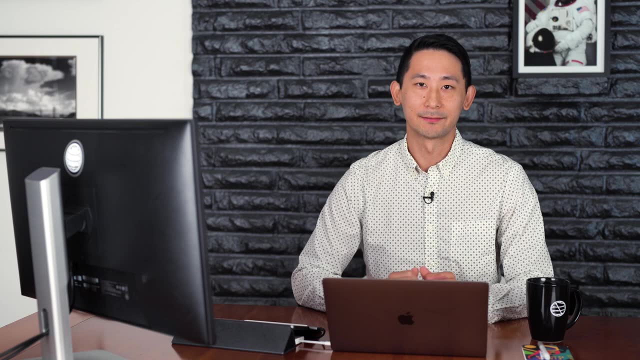 Today we're going to be learning how to install Qiskit and use a very specific circuit library in order to build our first quantum algorithm. In order to access this library, we're going to have to install Qiskit locally first. So let's go through really quickly how to do this. 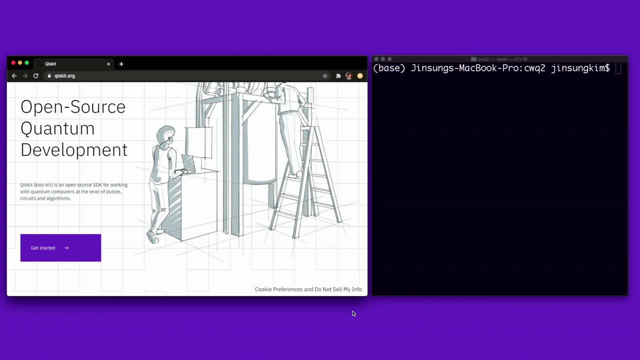 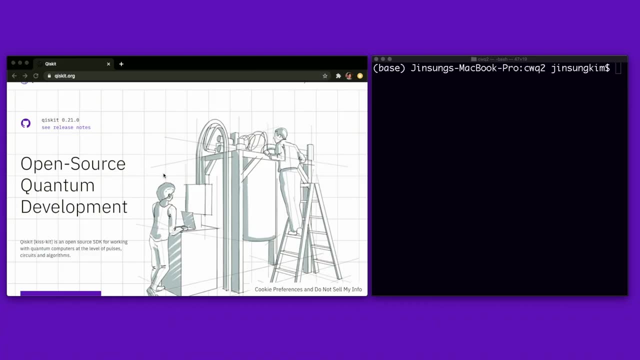 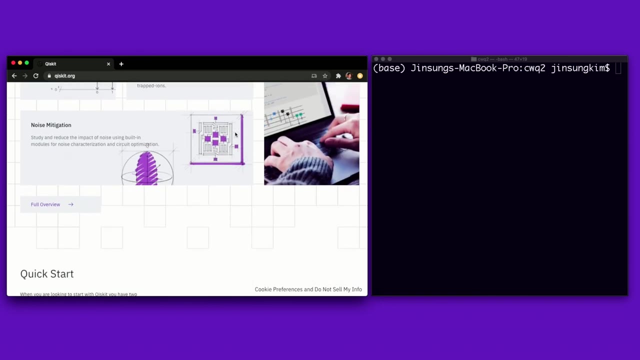 So Qiskit is an open source SDK used for programming quantum computers using Python, And don't worry if your Python skills aren't there yet- we'll work through things slowly. So the first thing I'm going to do is navigate to Qiskitorg. This will tell me exactly how to install Qiskit on my machine. 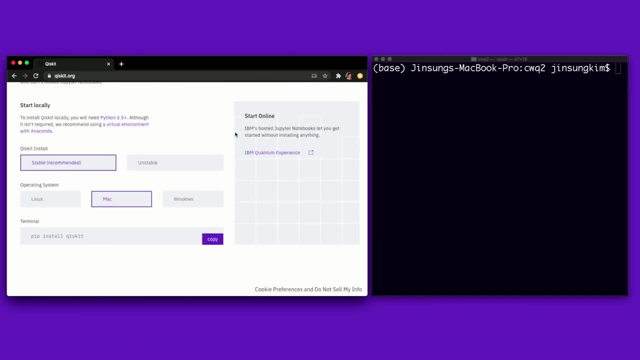 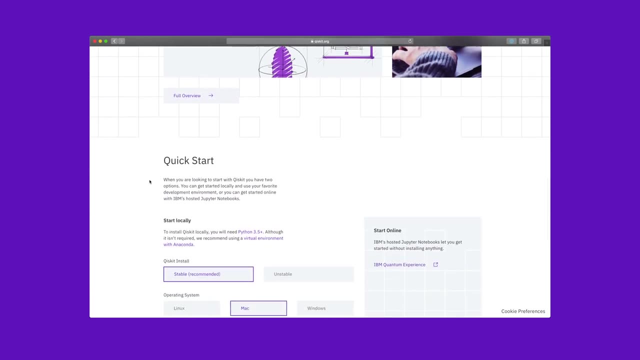 And there's generally two options for running Qiskit. You can either run it on IBM's hosted Jupyter notebooks or you can install it locally, And the first thing I want to do is if I don't have Python installed yet. 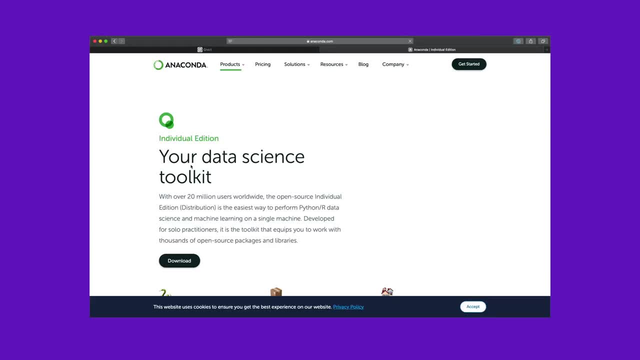 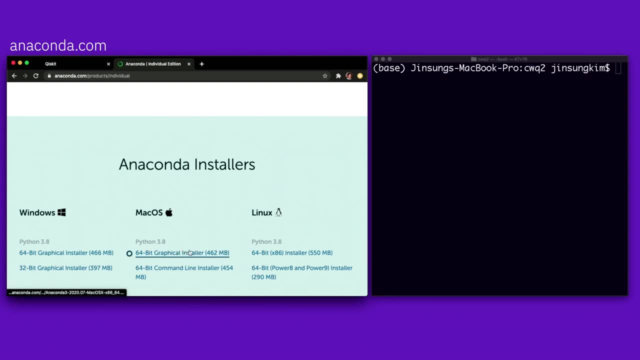 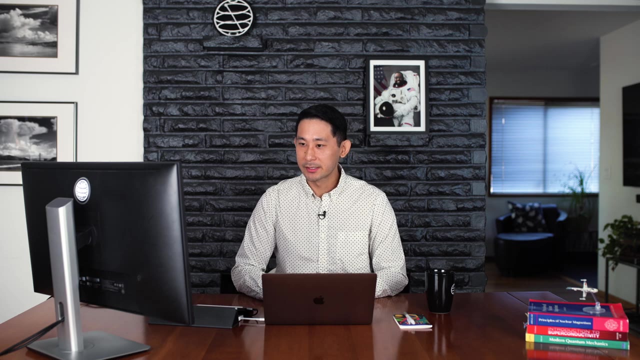 is to just install Anaconda And this will install all the things I need for Python. Click download. I have a Mac, so I'll just do the 64-bit Graphical installer And download And, like always, if you have a Windows or a Linux, just choose the appropriate downloader. 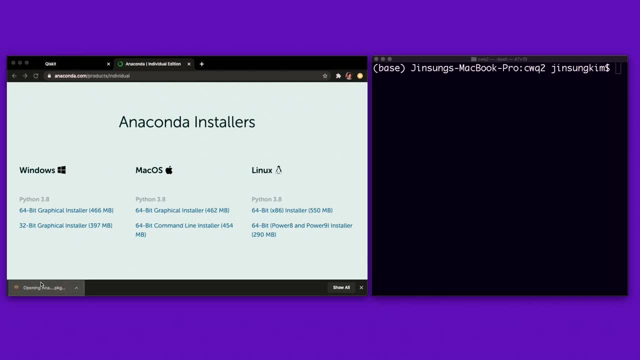 Okay, so now that Anaconda has downloaded, I'll just open this up And I'll install. So what I'm going to do first is set up the Qiskit library, And then I'm going to go ahead and install it. 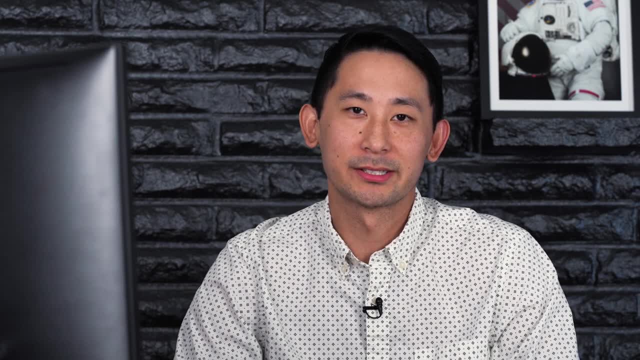 So what I'm going to do first is set up the Qiskit library, And then I'm going to go ahead and install it. So what I'm going to do first is set up my Python environment, which just is a good way for me to organize my Python packages. 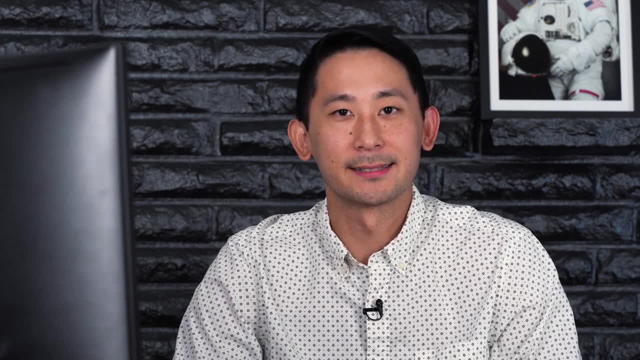 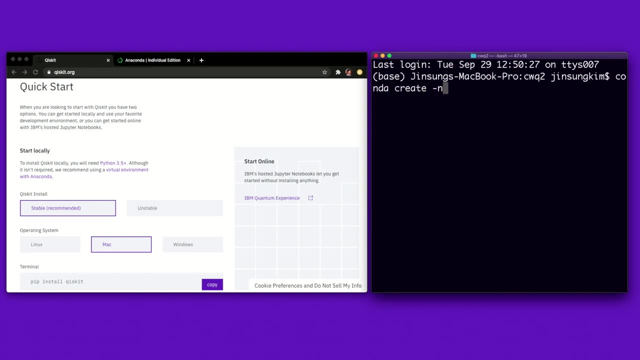 so that I have all the correct versions of all the packages in one place. So what I'll do is conda create dash n name of my environment, which will be coding with Qiskit or CWQ. I'll set my Python version equal to three and the Anaconda distribution. 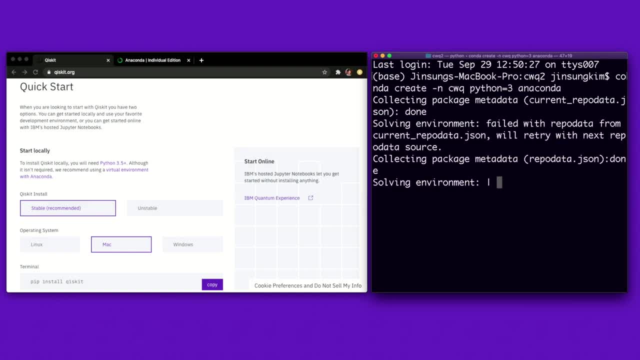 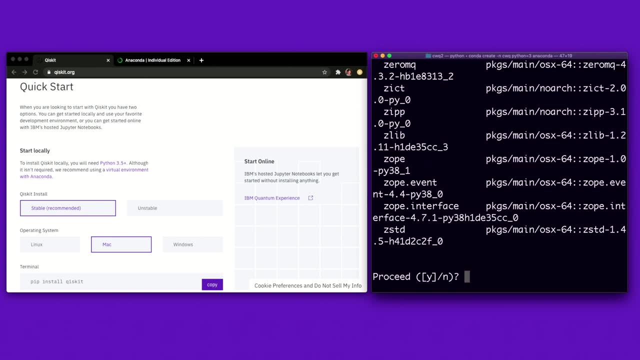 And I'll just create another D Тут over here. Okay, And I'm just going to watch this little thing spin. Okay, now it's done. Okay, So i'm going to proceed. Yes, And now that thing is going to spin some more. 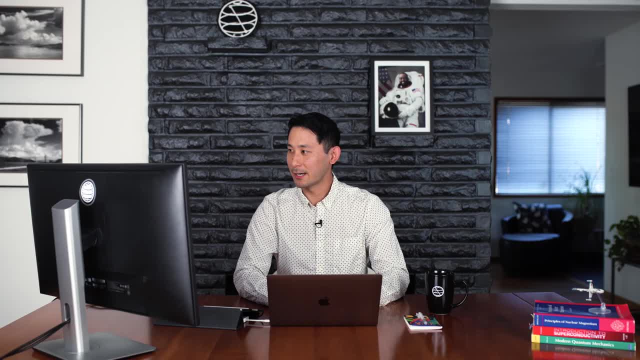 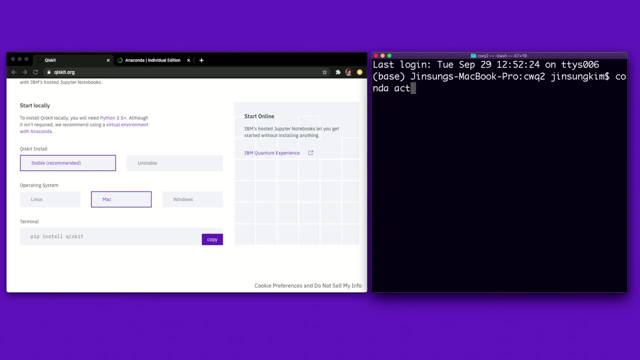 Okay, this might take a minute. So now that I have my environment setup, I'm going to enter my environment by going to Conda, Activate, The name of my environment, which is coding with Qiskit, with Qiskit, And I'm going to now install Qiskit into my environment. So from the Qiskitorg site. 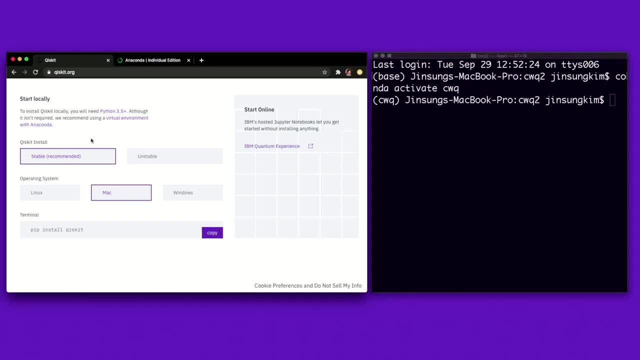 just following these instructions: start locally. I'm going to choose the Qiskit stable installation. I have a Mac, so I'll choose Mac, but it's the same if you have Linux or Windows. Just choose the correct distribution And then I'll copy this and pip install Qiskit into my environment. 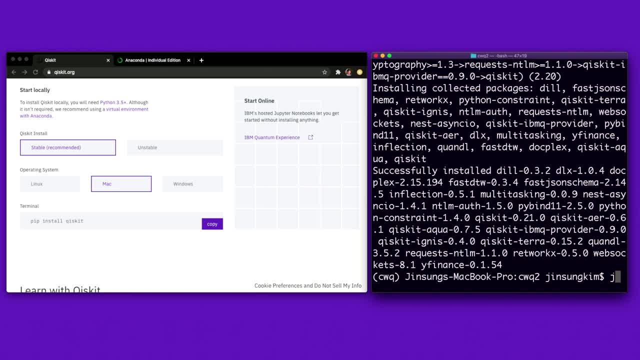 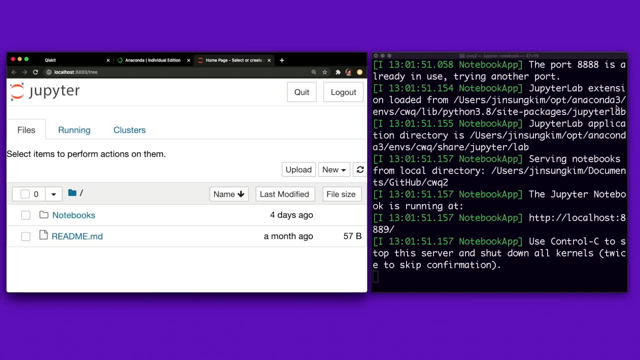 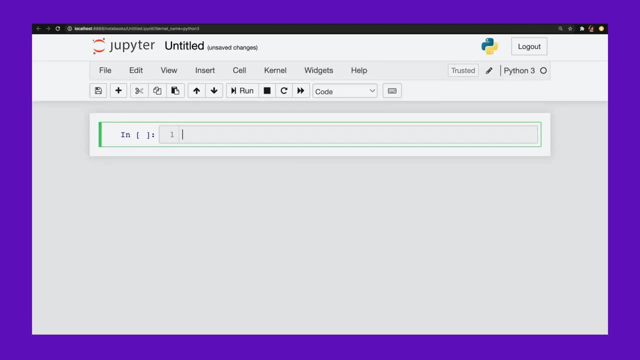 So now I have Qiskit installed and I'm just going to open up a Jupyter notebook so we can get started with our algorithm. Perfect, So I'm going to open up a new Python 3 notebook and let's get started with our algorithm. 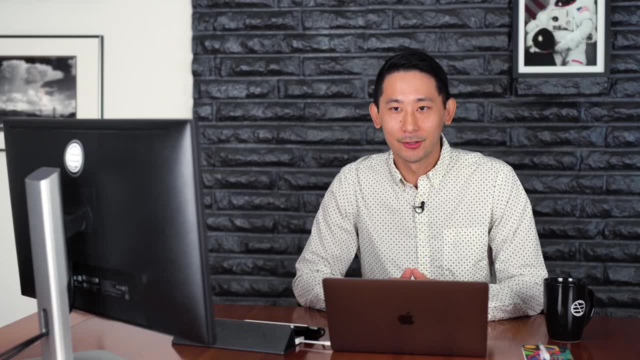 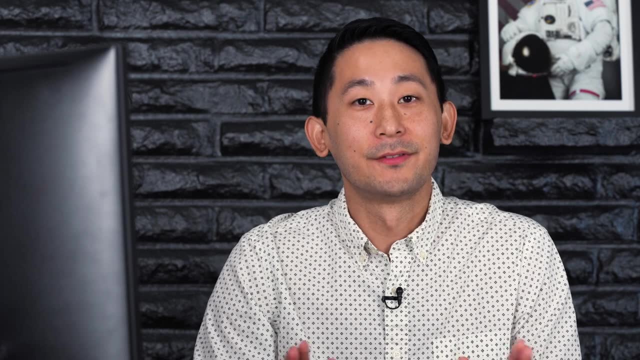 So let's build our first algorithm. So let's build our first algorithm from the circuits library. now, In order to do this, we need a few parts, some data to input, a circuit to run the calculation and then an output. In physics, we often talk about signals, and signals represent the transmission of information. 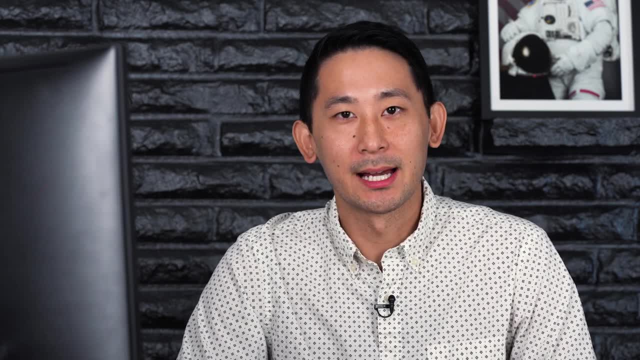 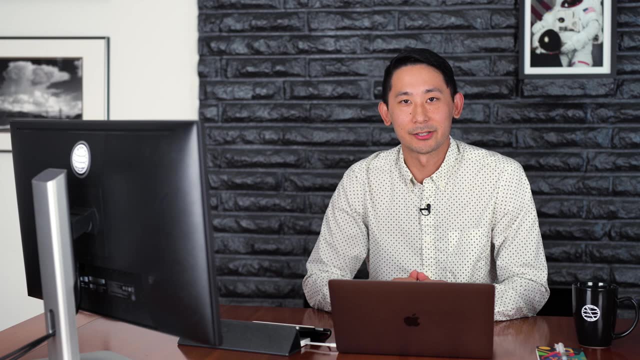 And generally we use bases or units such as frequency or time to represent what kind of information that we're transmitting. I'm going to show you a quick example of an algorithm that's already built in Qiskit circuit library, called the Fourier checking circuit. 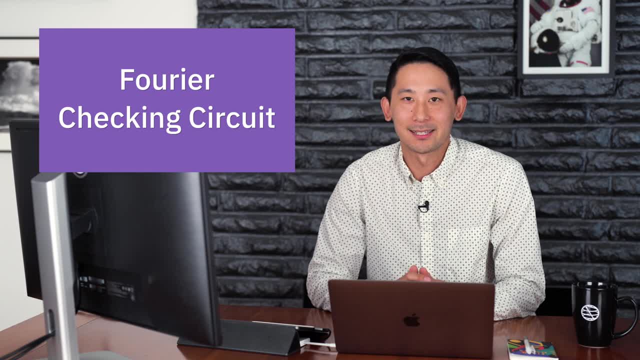 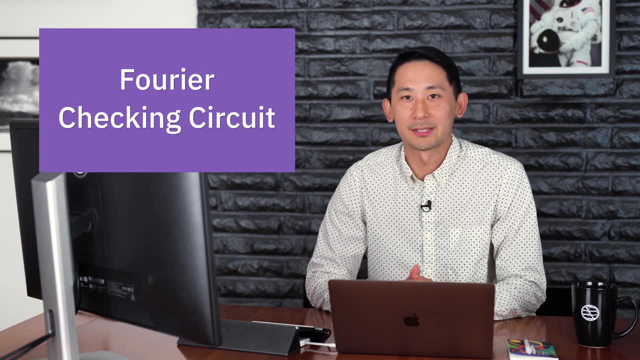 The Fourier checking circuit is an important tool used in the signal process, signal processing domain and is a fundamental circuit used in many other quantum algorithms, For example Shor's algorithm, which we'll cover in a future episode. These circuits can be run on a real quantum backend or on 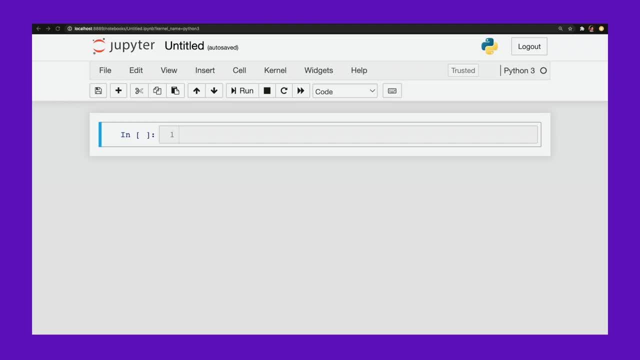 one of the high performance simulators that are available through Qiskit. All right, so let's get started with the algorithm. So the first thing I'm going to do is do my imports. So I'm going to import Qiskit quantum info as QI and this is going to be doing the calculation. 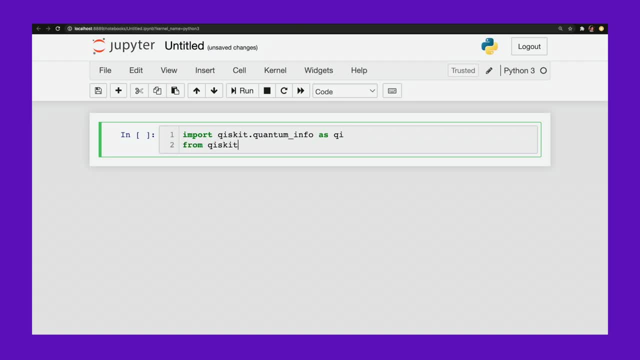 I'm going to import from the circuit library the Fourier checking circuit And I'm going to import my visualizer, Qiskitvisualization. import plot histogram: Okay, shift, enter to execute that This algorithm. I'm going to define two functions. They're just lists. 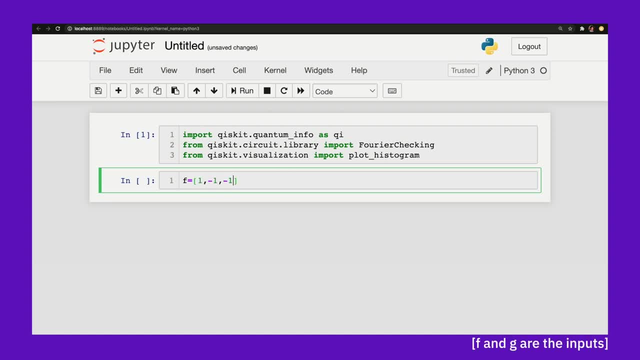 F is equal to 1 minus 1 minus 1 minus 1.. And G is equal to 1: 1 minus 1 minus 1.. So now that we have our two functions, F and G, the Fourier checking circuit will tell us. 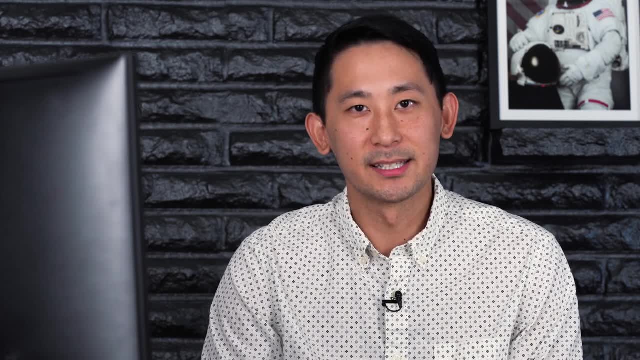 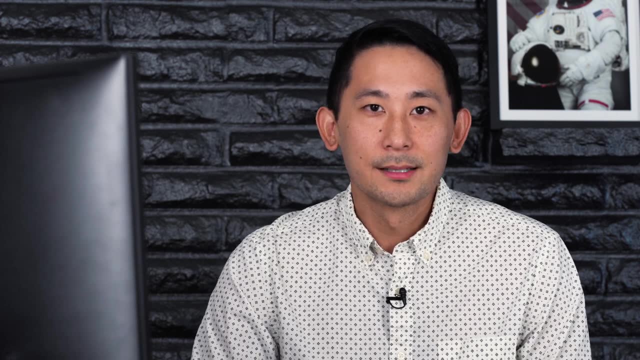 how correlated the Fourier transform of G is to our function F, And it turns out that a quantum computer can perform this calculation much faster than a classical computer can. So the circuit will output a probability for the 0,, 0 state And if the probability is greater than 0.05,. 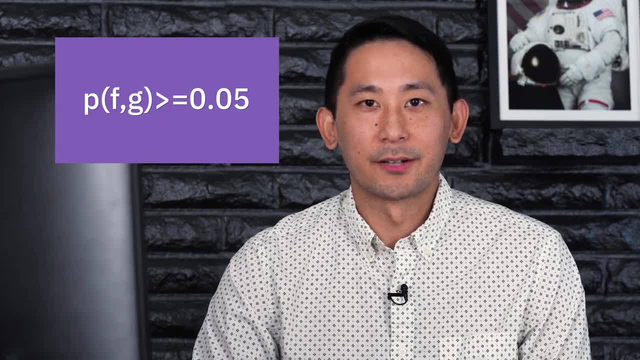 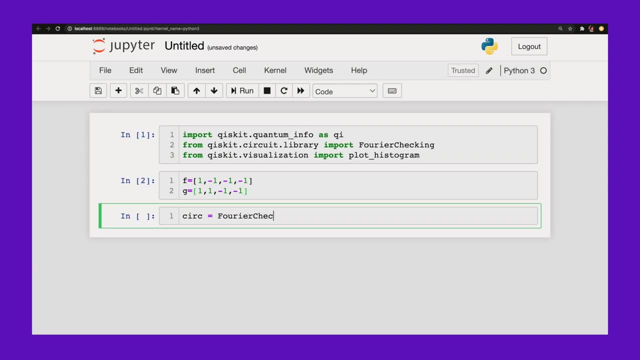 then the Fourier transformer of our function G is correlated with our function F. Okay, so I'm going to set up my circuit equals Fourier checking and I'll put in my two functions: F is equal to F and G is equal to G. Okay, do circdraw, see what this looks like. 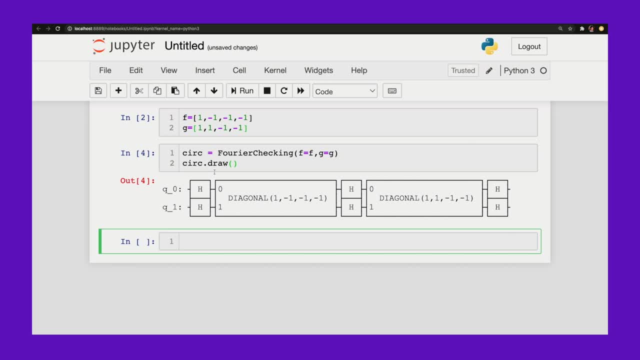 Okay, and this is what my quantum circuit will actually look like. So let's run this: 0 equals qistateVector from label 0, 0, going to evolve this state vector is equal to 0.evolve my circuit and I'm going to get my probabilities back here. 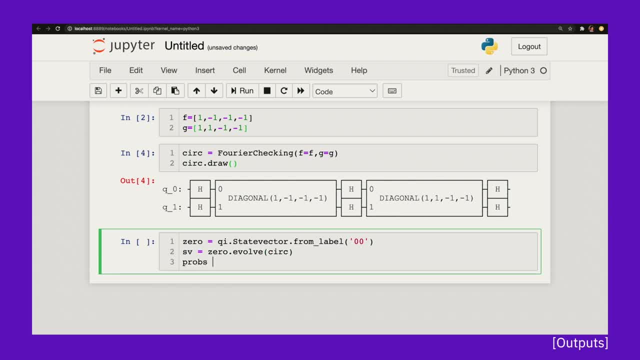 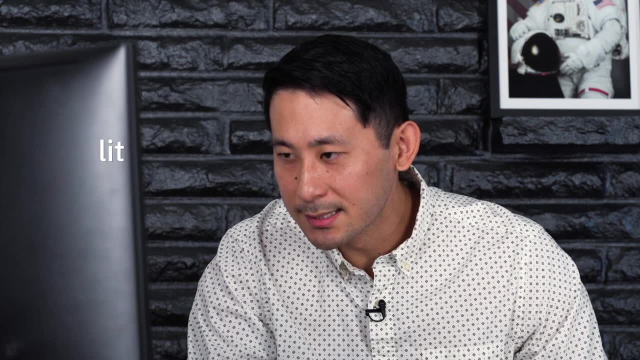 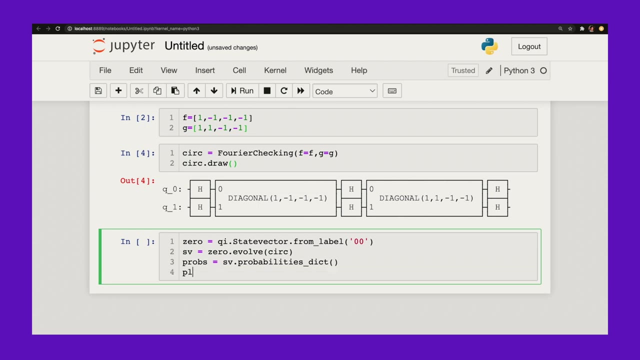 ProbstateVector is equal to 0.evolve Equals: svprobabilities, probabilities, probabilities. Okay, and then I'm going to plot what this looks like And remember I'm only interested in the 0, 0 probability. Okay, perfect.